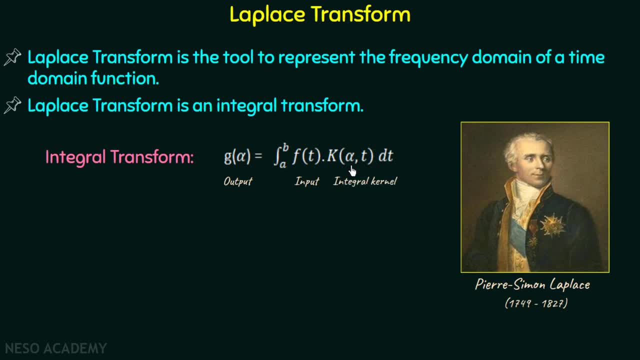 And k of alpha comma t is the function of both alpha and t, and that's why we call this function as integral kernel. So we can see that the integral kernel is a function of both the input variable and the output variable. Moving on to the next point, the Laplace transform, 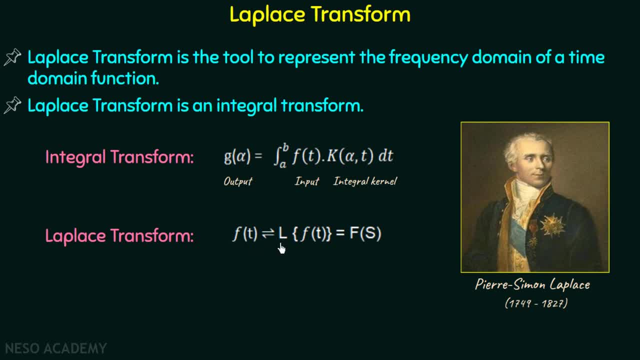 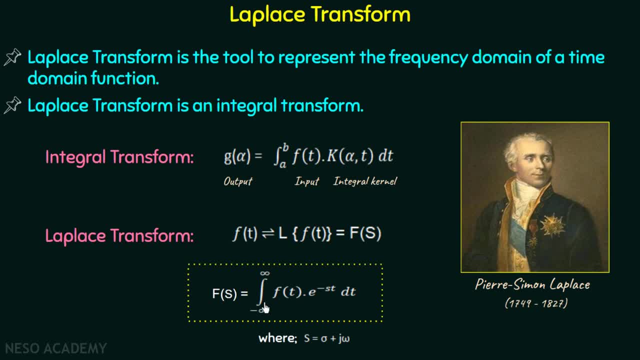 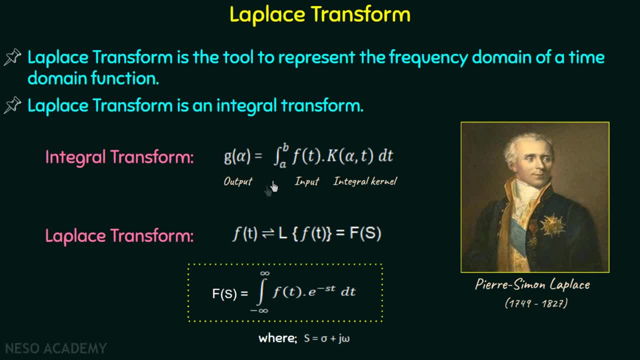 this expression with the general integral transform expression, we can see that f of s is the function of s and this is the output, f of t is the function of t and this is the input. and e to the power minus st is the function of both s and t and we can call this function as the integral kernel And this is the Laplace. 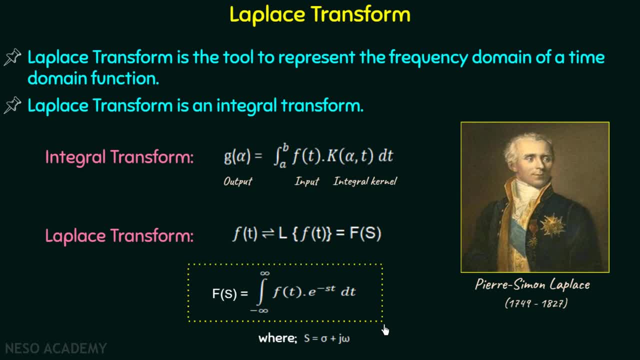 transform expression which is used to convert the time domain function to a frequency domain function. In this expression, s is equal to sigma plus j, omega, in which the sigma is the damping factor of control system. the stability of control system depends upon the damping factor and the omega is angular frequency. So now we are done with the expression of. 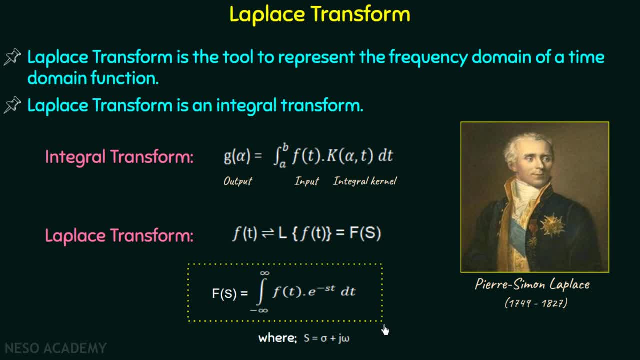 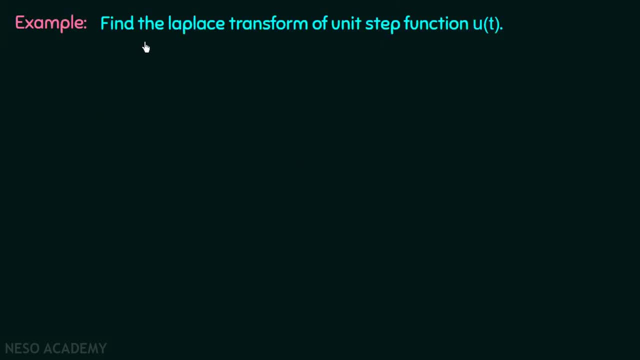 Laplace transform. We will now use this expression to convert a standard time domain signal to its frequency domain. Let's take an example: Find the Laplace transform of unit step function u t. Moving on to the solution we are given, the value of f of t is equal to u t and we: 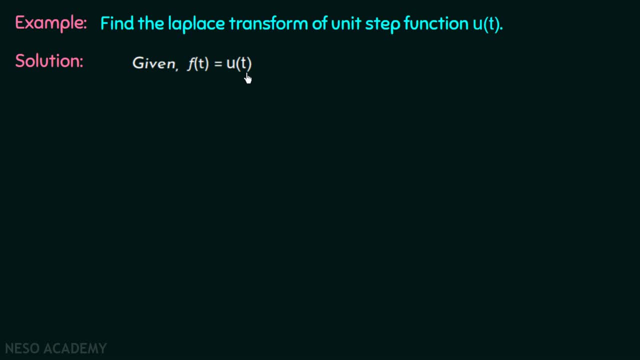 need to find its Laplace domain From the definition of unit step function. we can say that unit step function is equal to one when t is greater than zero, and it is equal to zero when t is less than zero. We can also plot this function graphically like this: 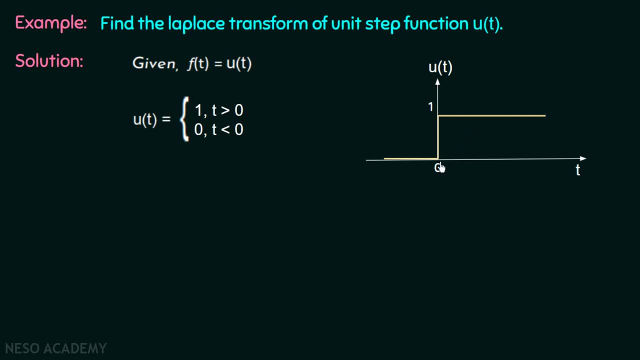 Whenever t is greater than zero, the value of function is one, and when t is less than zero, the value of function is zero. So, on the right half plane, the value of the function is one and on the left half plane, the value of the function is zero. We will now calculate. 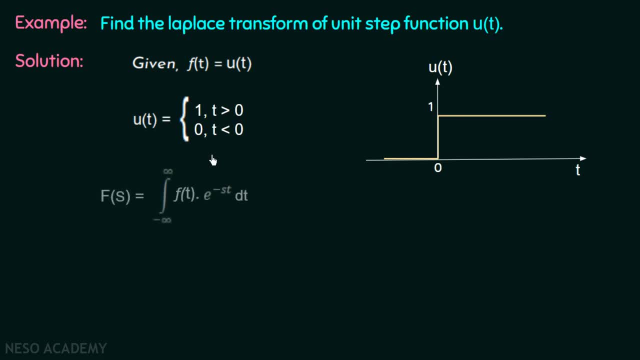 the Laplace domain for this function. The expression for finding the Laplace transform is: f of s is equal to integral, from minus infinity to infinity. f of t multiplied e to the power minus st dt. Now we will replace this f of t by u t like this: From the definition of u t, we know that it is equal to one when. 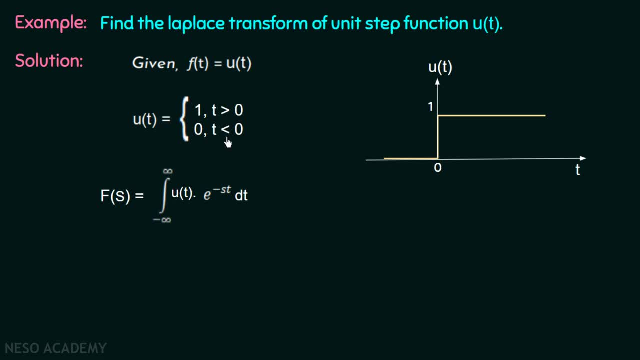 t is greater than zero and it is zero when t is less than zero. So the integral from minus infinite to zero will become zero because the function value is zero in the left half plane and on the right half plane the function value is one. So our integral limits will change from zero to infinite because the value 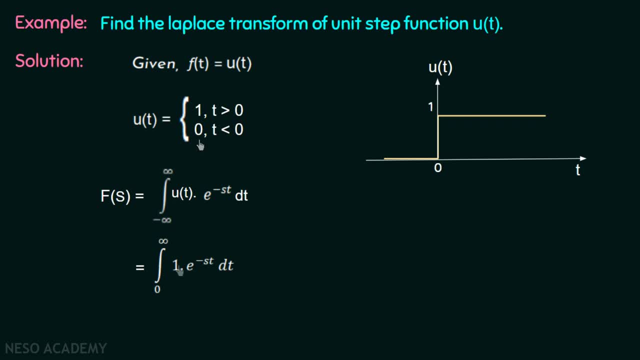 from minus infinite to zero is zero. So now we have this function and we need to integrate this function. So we know the integral of e to the power minus st. It is minus one upon s e to the power minus st and we have the limits from zero to infinite. 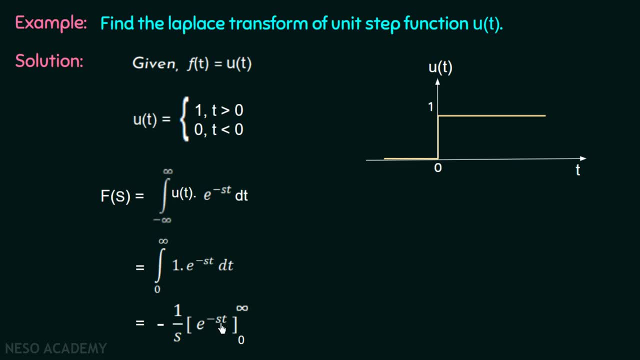 By substituting the limits, it minus of e to the power, minus zero will become minus one. So we will have minus one upon s multiplied with minus one and this will come out to one upon s. So finally we have got the Laplace domain of unit step signal and it is given as Laplace of u of t is equal. 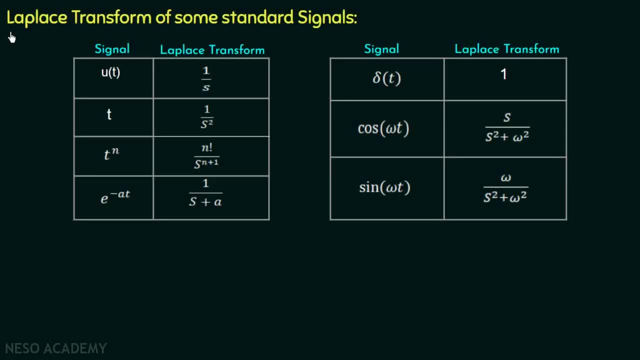 to one over s. So this is the list of Laplace transforms of some standard signals We have already seen. the Laplace transform of ut is one over s. The Laplace transform of t, or we can say the ramp signal, is one over s square. The Laplace transform of t to the power n. 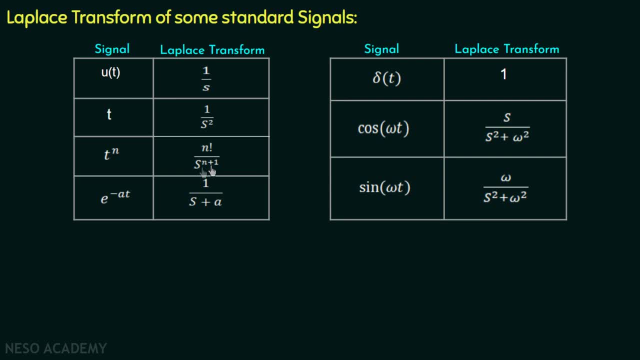 is n factorial over s to the power n plus one. The Laplace transform of e to the power minus at is one over s plus a. The Laplace transform of impulse signal is equal to one. The Laplace transform of cos of omega t is one over s plus a. The Laplace transform of 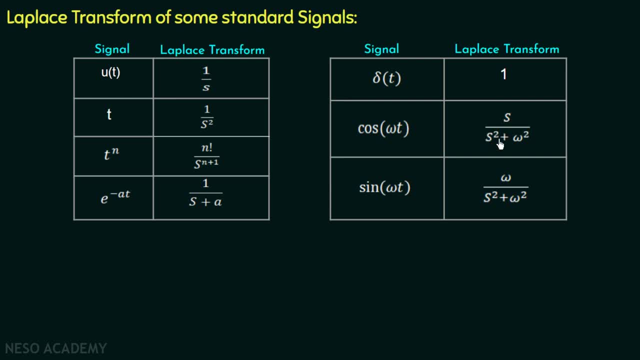 impulse signal is equal to one. The Laplace transform of cos of omega t is one over s plus a. The Laplace transform of impulse signal is equal to one. The Laplace transform of t is one over s square plus omega square. The Laplace transform of sin of omega t is: 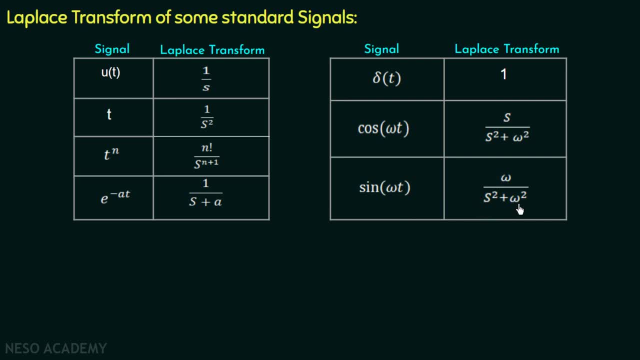 one over s square plus omega square. All these Laplace transforms can be obtained by the same expression. Now this will be your homework task: to derive all these Laplace transformations using the same expression. I will give you one hint for calculating the Laplace transform. 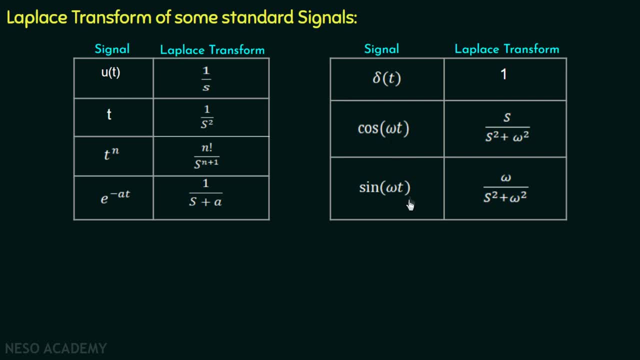 of these two functions, cos omega t and sin omega t. We use the complex conjugate property of sinusoidal function to calculate the Laplace transform of these two functions. We can write cos omega t as e to the power j omega t plus e to the power minus j omega. 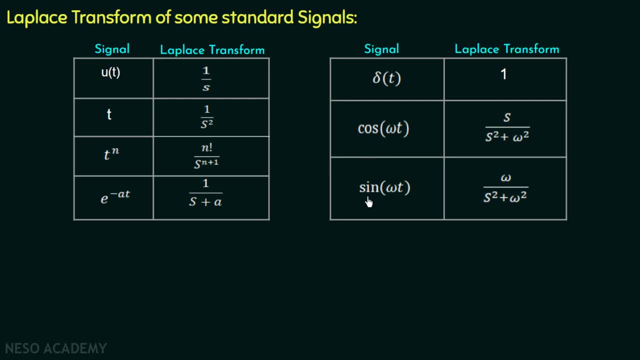 t over 2 and similarly, sine omega t can be written as: e to the power j. omega t minus e to the power minus j. omega t over 2j. So these are the hints to calculate the transforms of these two functions and this will be the 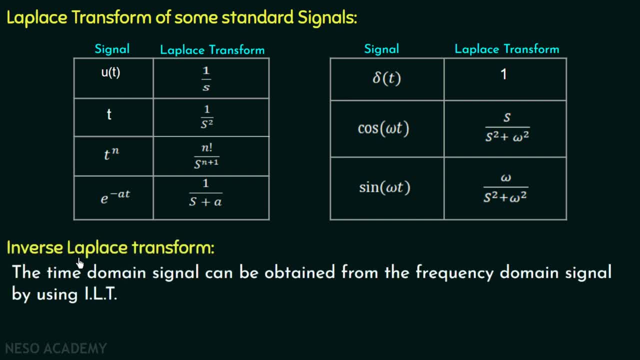 homework for you. And now we will move on to the inverse Laplace transform. So, as the name suggests, inverse Laplace transform is the inverse of Laplace transform. So from the Laplace transform we can get the frequency description of a time domain. 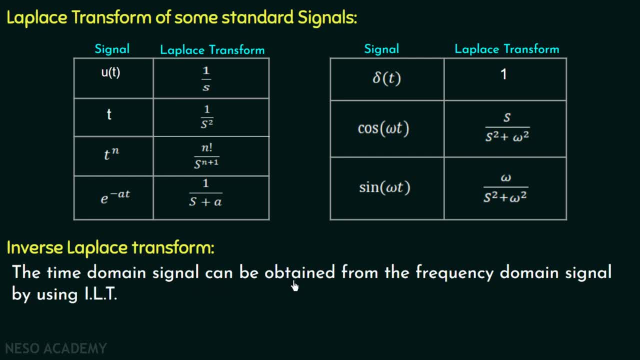 function. Similarly, the time domain signal can be obtained from the frequency domain signal by using inverse Laplace transform. The expression of inverse Laplace transform is given as: f of t is equal to 1 over 2 pi j integral from sigma minus j omega to sigma plus j omega. f of s multiplied. 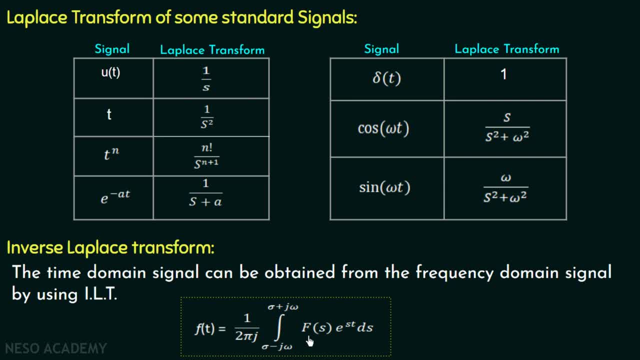 e to the power st ds. So here in this expression the input is the frequency domain function and the output is the time domain function. But we will not use this complicated equation to find out the inverse Laplace transform. We will find the inverse Laplace transform by using the method of partial fractions. 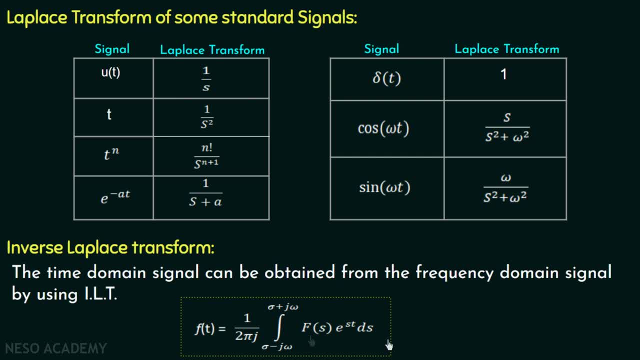 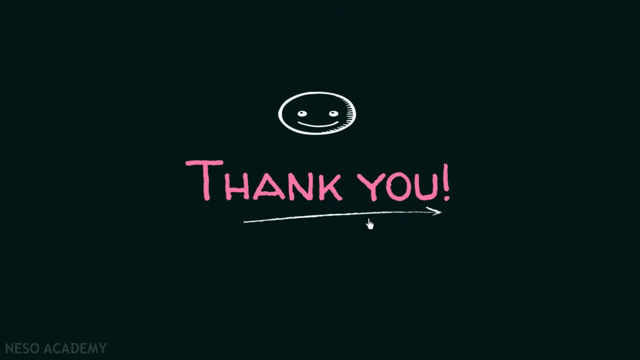 The method will be clear to you when we will take some examples. So now we are done with this lecture. In the next lecture we will take some properties of Laplace transform. Thank you for watching this lecture. I will end this lecture here. See you in the next one.